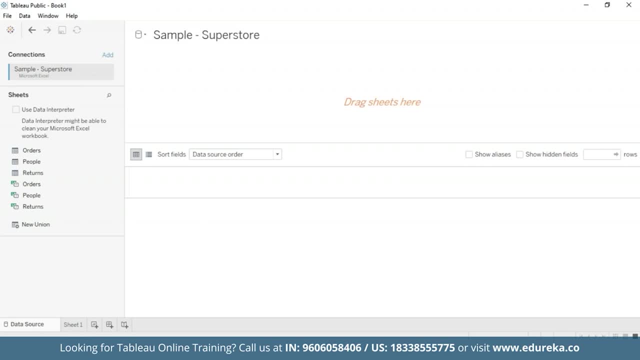 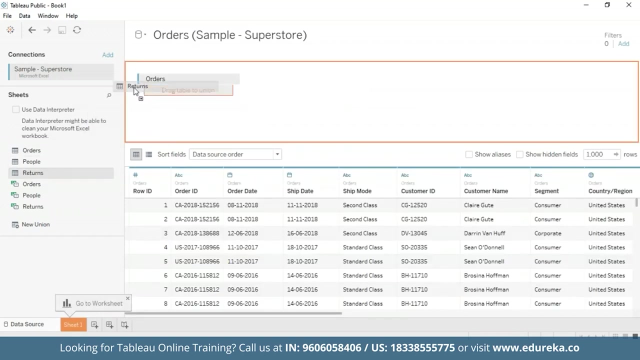 prepare the data. First, we need to left join the returns table to the orders table. So let's go ahead and do that. I'm going to drag the orders table And the returns table as well Here. I'm going to click on this icon and select left join. 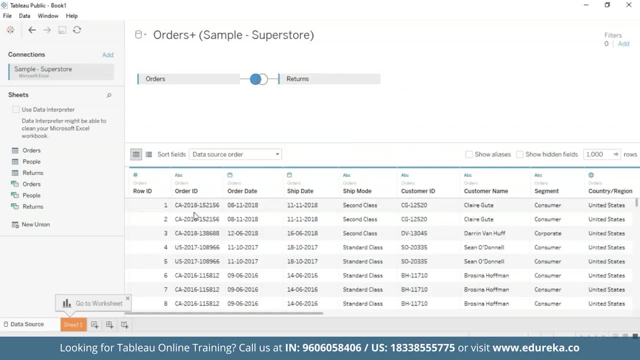 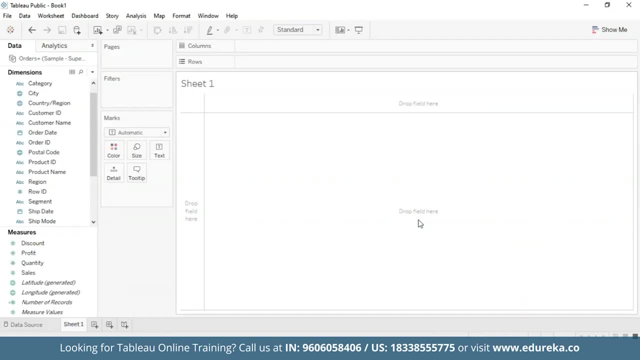 And then I'm going to go ahead and close it. Next, what we're going to do is we're going to go straight to our sheet- All right, and create a calculated field to count the number of returns, All right. So we're going to go to analysis on the main title bar and select create calculated field. 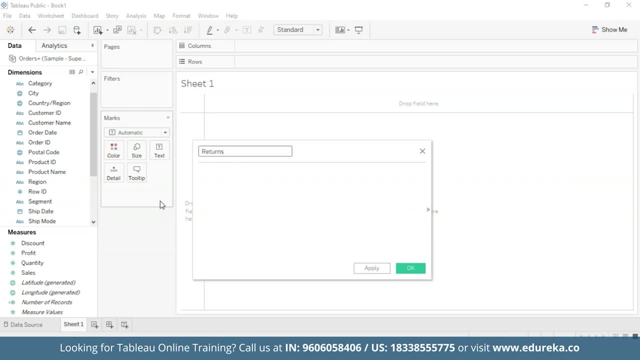 Let's name this- returns, which will be true to its purpose, And we're going to use a function known as count. Here. we're going to count the returned subcategories, And now it shows us at the bottom That our calculation is valid. So now we are all set to build a Pareto chart. Now you can. 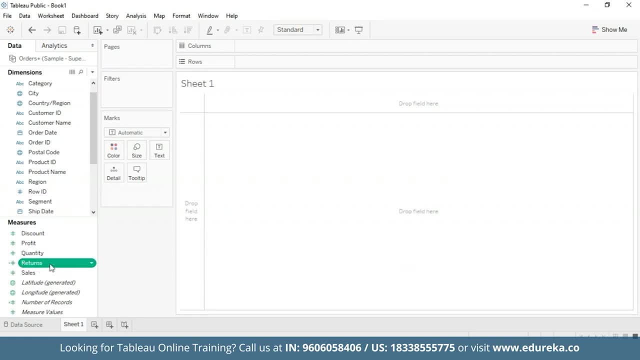 see that our returns measure is available in the measures pane. We're going to first start by creating a bar chart that looks at the number of returns per product subcategory And then we're going to sort it in descending order. So I'm going to go ahead and create a bar chart And then we're going to sort it in descending. 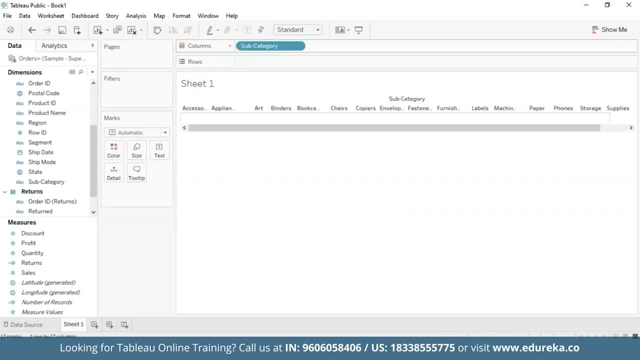 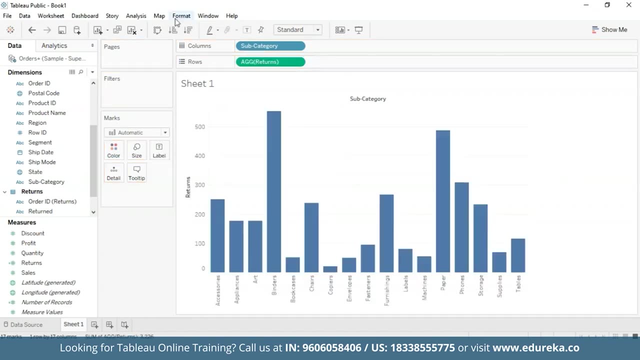 order. So I'm going to go ahead and create a bar chart And then we're going to sort it in descending order. So I'm going to bring the subcategory to the columns and return to the rows, And then I'm going to sort it in a descending order. Next, what I'm going to do is go ahead and create. 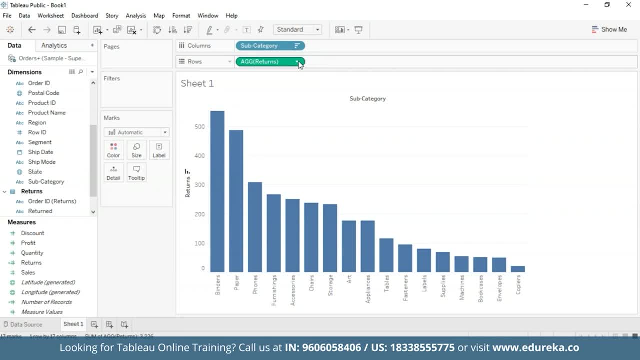 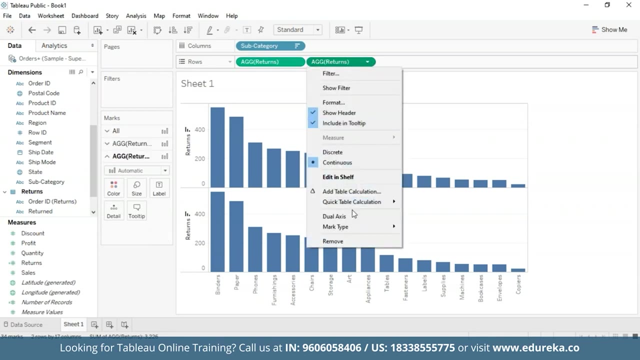 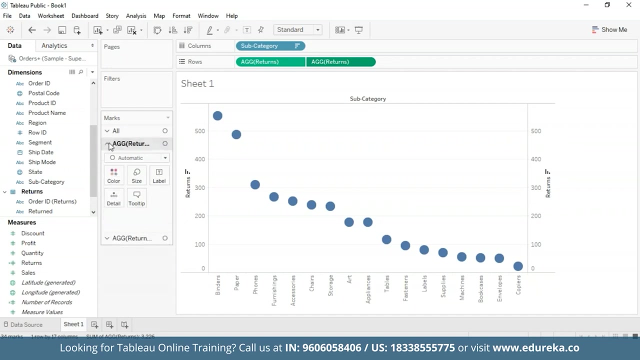 a dual axis combination chart, which I'm going to do in my rows. For that I'm going to drag the returns measure again to my row shelf, bring it over here And click on the drop down button and select dual axis. I'm also going to go on the left. 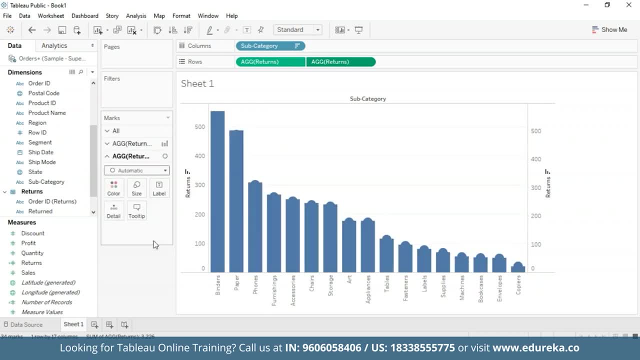 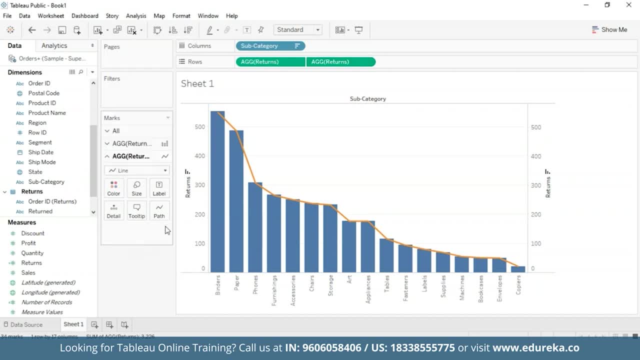 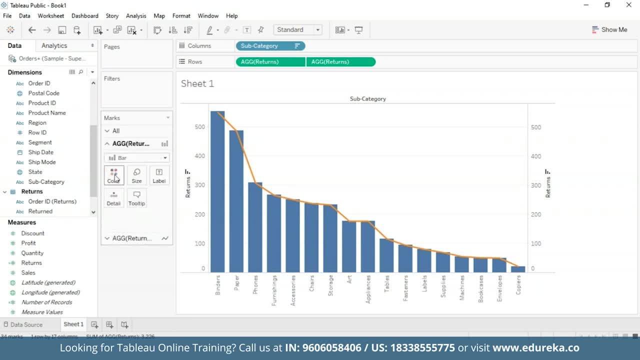 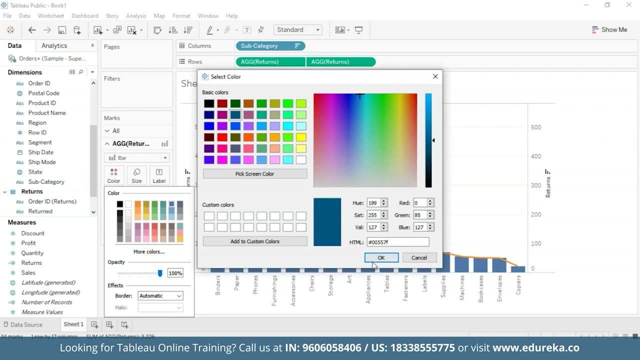 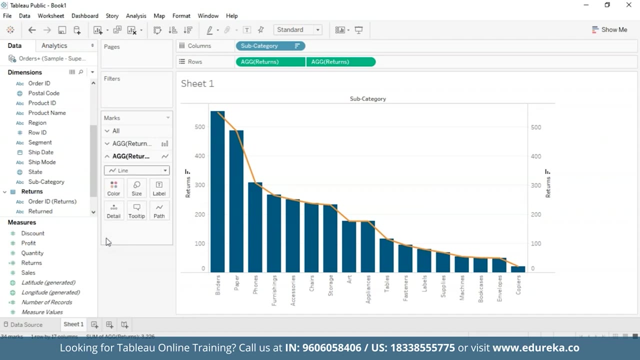 the screen. I'm also going to go and change the color of the bar chart to something deeper For visibility purposes. Okay, Yeah, this color looks good. Okay, Now the step that makes a Pareto chart. a Pareto chart is basically adding a table calculation and a section to 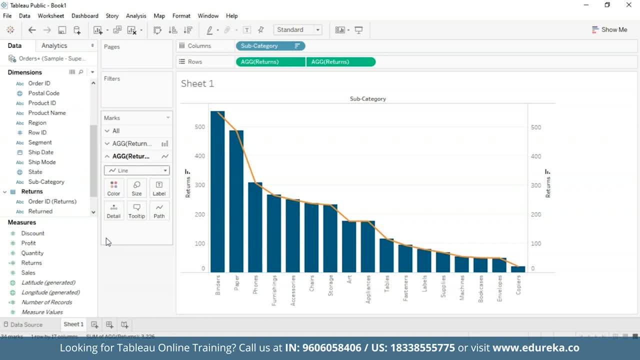 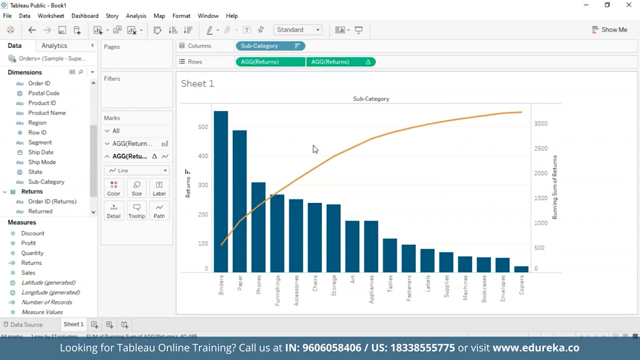 the table calculation and a secondary table calculation to this return spill. They shall display the cumulative percentage of returns across products in different subcategories. Now to do that: first, upon right-clicking on the second panel, we get quick table calculation option, and I'm going to choose a running total at this point. a chart should look something. 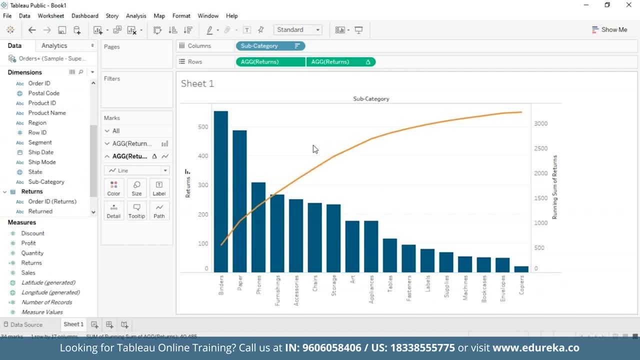 like this: now, with the table calculation for running total, You can add a second table calculation to the result and that is how we are going to be calculating the raw running total number for each product subcategory, and then we'll add a secondary calculation to determine the cumulative percent total. now for addition. 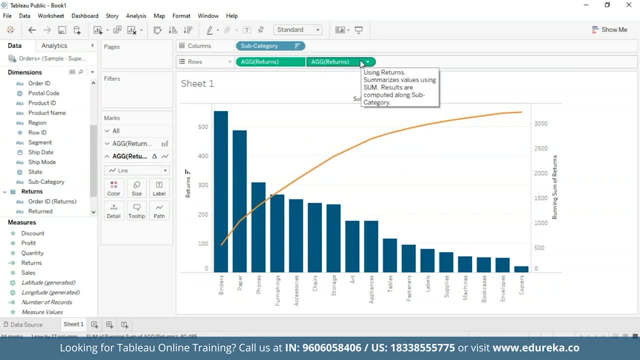 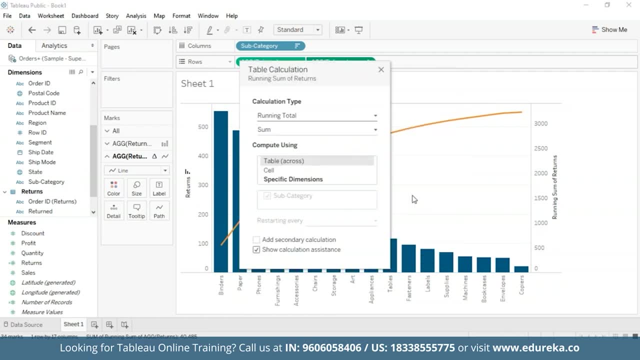 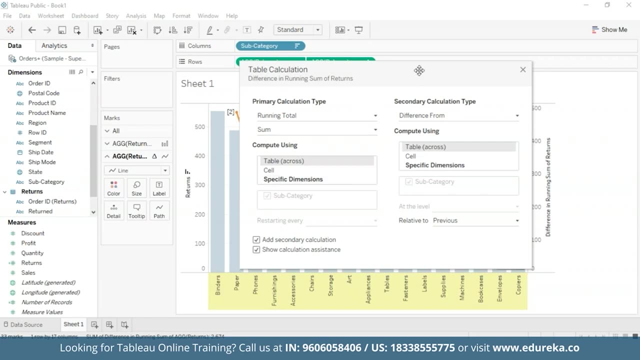 of a second table. I'm going to go back to the return spill, Go to edit table calculation And check this box in the bottom that says add secondary calculation. Okay, I'm just going to move it a little bit to the center, Okay. 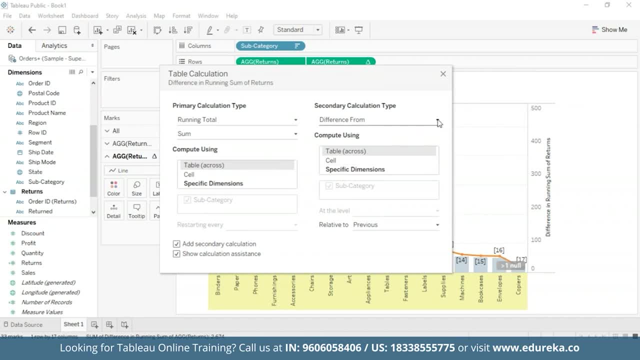 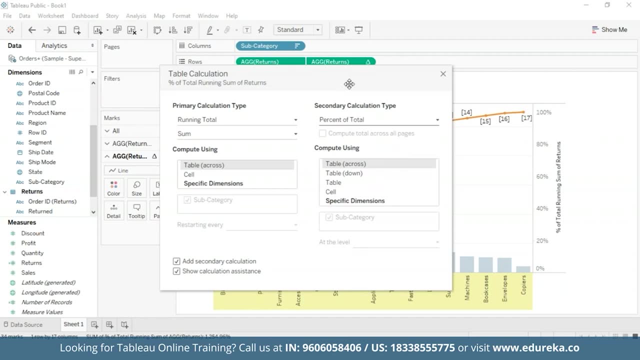 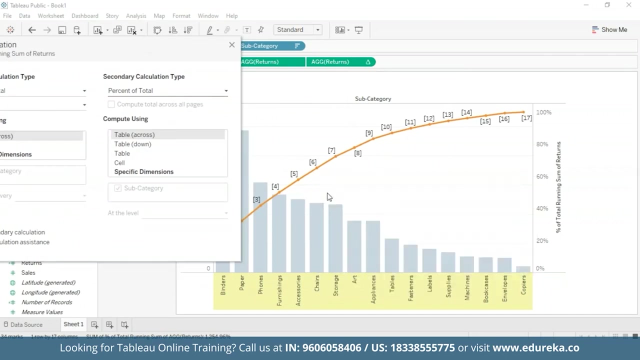 Now, this is my secondary calculation type, and here I'm going to switch it from difference from two percentage of total, percent of total. All right, at this point, if I move this dialog box, your graph should look something like this: This is basically the cumulative percent. 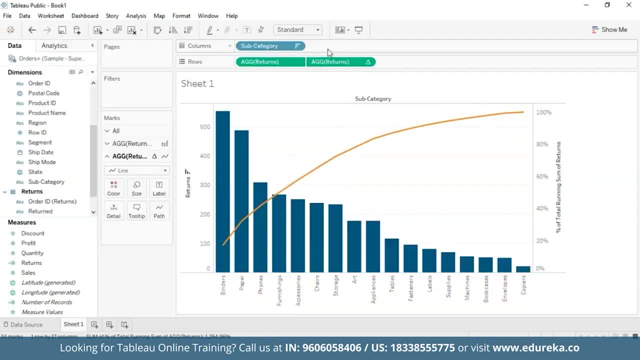 of total. Okay now, after changing the access tick marks for a cleaner look, you will be left with this following visualization that you see in front of you. wasn't that difficult, was it? you know for a fact. now, by hovering over this, you'll get your subcategory: the percentage of total. 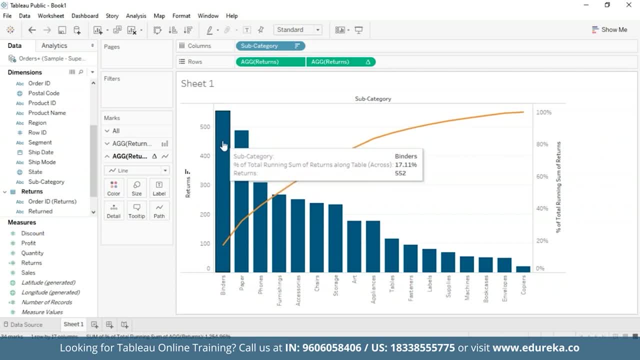 running sum of returns and the total number of returns or subcategory. So, as we can see, right now, 17% of all binders Does come back, which is terrible for a company and will bring a lot of loss for a company dealing with office supplies. Now this Pareto chart and tableau can now be used for drawing. 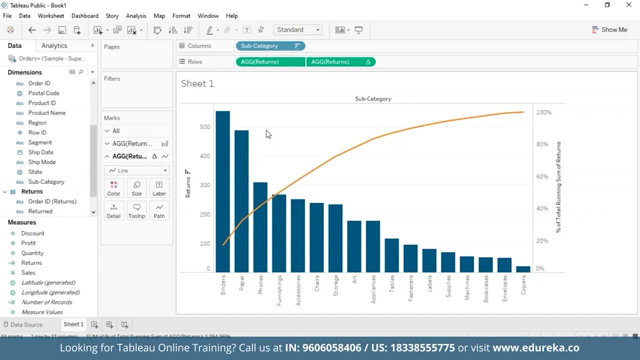 insights such as the businesses three most return product subcategories, causing about 40% of the total returns, which you can see: our binders papers and phones. Pareto charts are usually a very effective way to quickly highlight potential for improvement and give enterprises a scale. 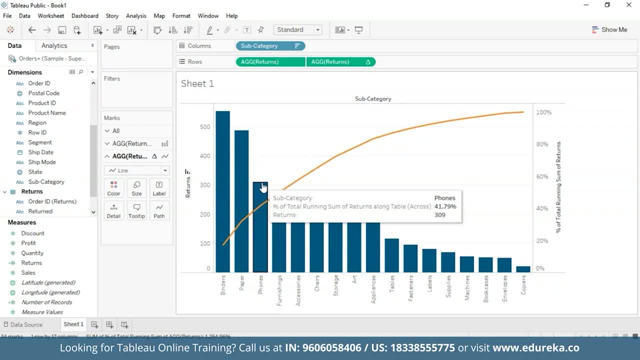 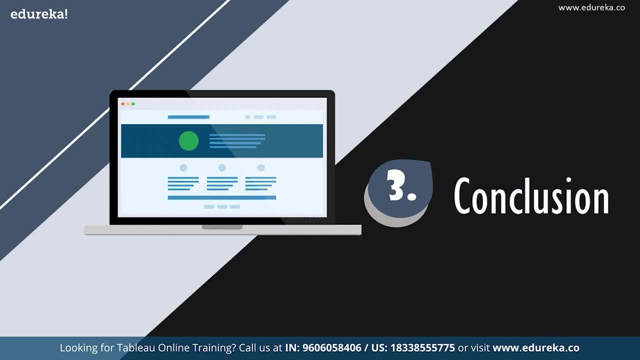 For how urgently a quality control problem should be treated. with that, I come to conclude my session now. a downside to Pareto chart is that it can only show qualitative data that can be observed. It merely shows the frequency or an attribute of measurement. one disadvantage of generating Pareto charts is that it cannot be used to calculate the average. 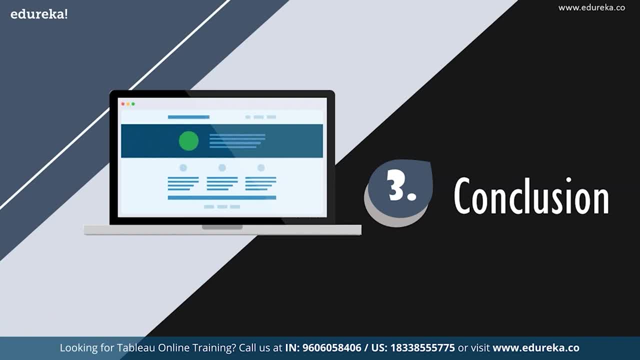 of the data, its variability or changes in the measured attribute over time. the main function of Pareto analysis Is to discover the causes of events or to quantify the relative frequency of when these events occur. Pareto charts are powerful tools for solving business problems because every 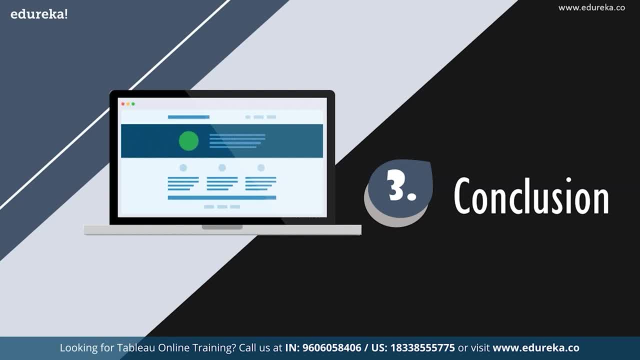 process produces defects, mistakes and errors, and hence the need of qualitative analysis. a Pareto chart or a diagram analyzes the frequency of problems or causes of problems in a process, and this technique works wonders to find out the reason for your loss. I shall leave you with that thought in mind. with that, I come to the end of this mini session.